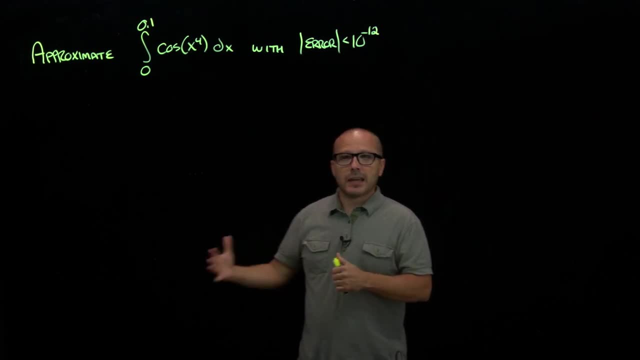 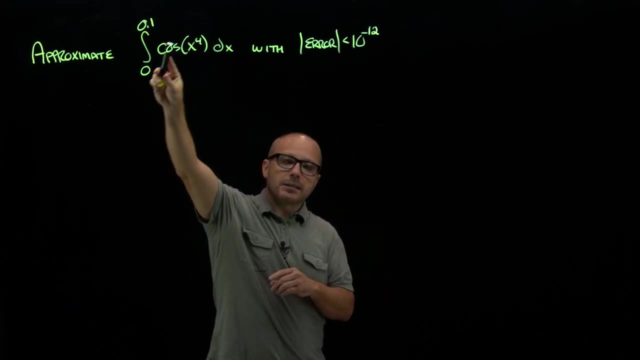 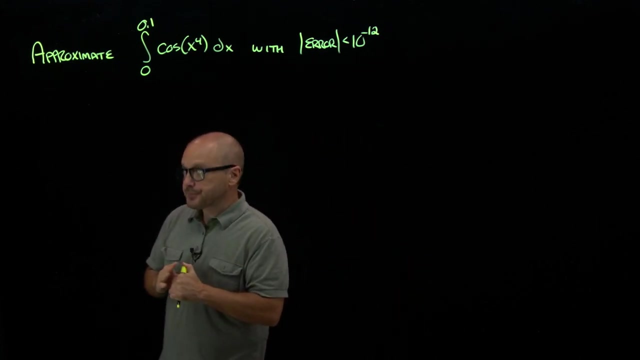 So we, we'd like to avoid that. Let's assume we can't do infinite precision calculation on each one of those points. What could we do? And what I want to do is replace this function with its Taylor series. So let's remind ourselves, first of all, cosine. We know now that cosine x is. 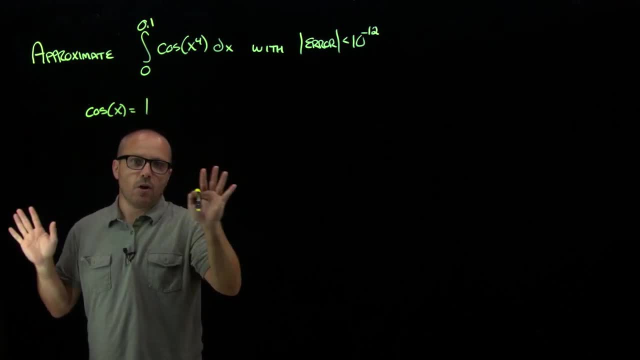 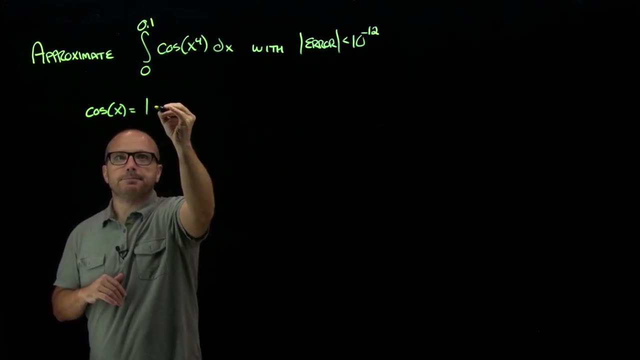 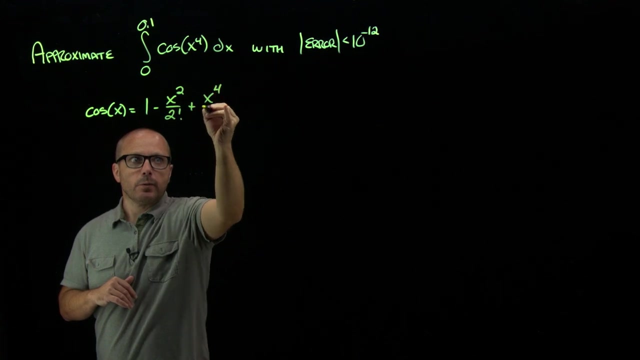 identically equal to its Taylor series everywhere, right, For all values of x. So we could really do this on any interval, because it's always true: Cosine x equals its Taylor series, And I'm not going to write sigma notation From what we're doing, I think. 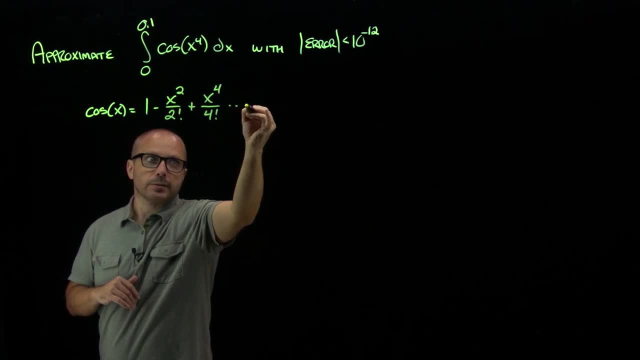 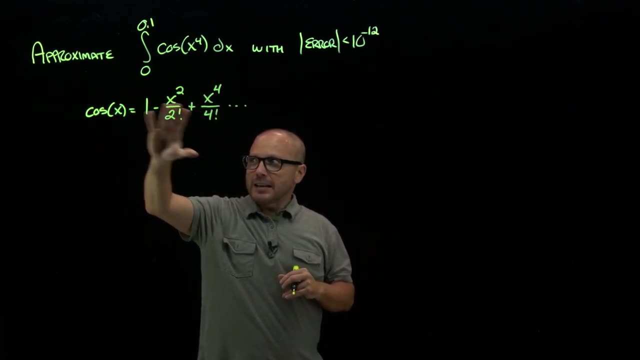 it'll be easier to follow if we just write out terms and then dot, dot, dot, right. So I am within my rights to interchange these two statements anytime I want. So that means, if this function equals this, when I plug in x to the 0, I'm going to get x to the 0.. So that means, if this function equals this, when I plug in x to the 0, I'm going to get x to the 0.. So that means, if this function equals this, when I plug in x to the 0, I'm going to get x to the 0. 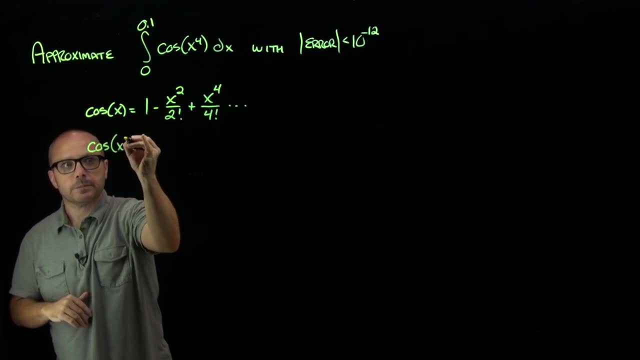 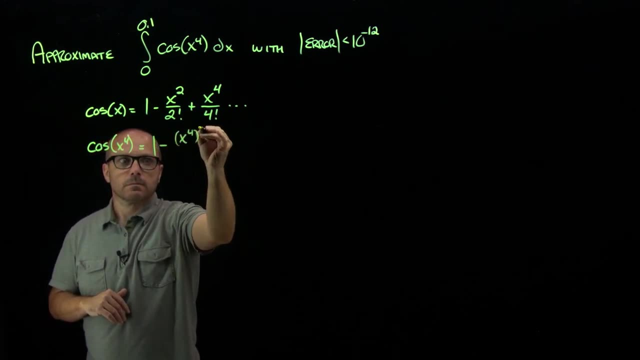 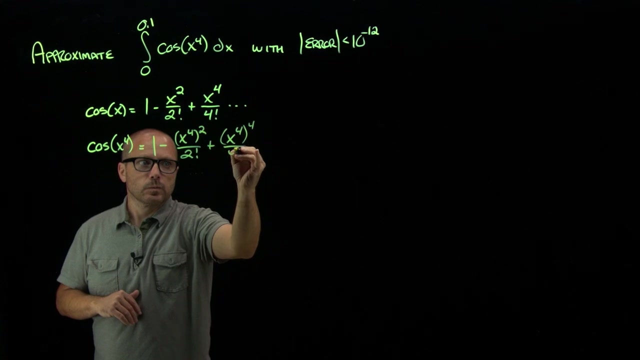 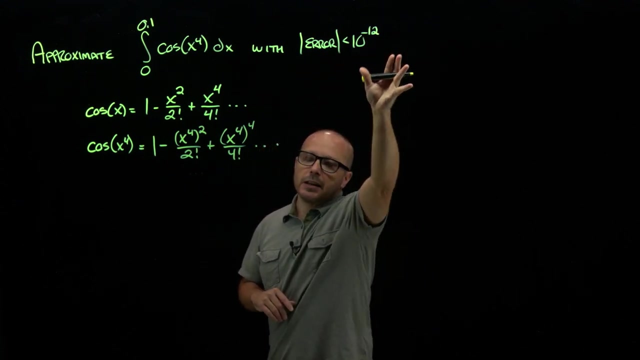 And if we do that and say exit 4 on the left, it should be equal to plugging in x to the 4th on the right. Now I set an error bound of 10 to the negative 12th, just as a sort of arbitrary. 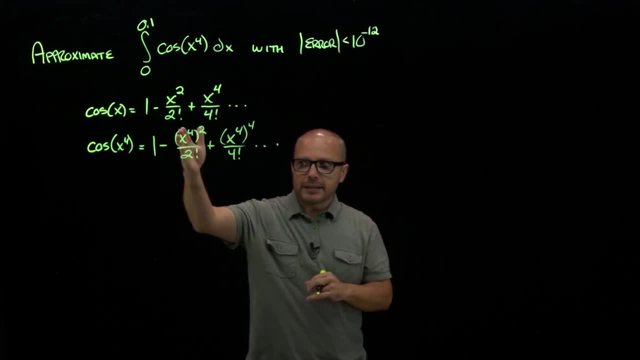 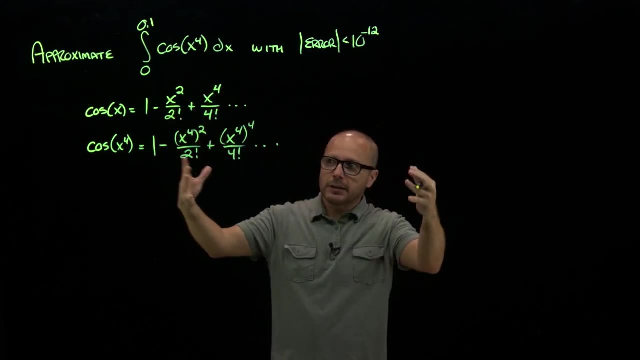 fairly small value there. I don't know how many of these terms we're going to actually use When we finally get down to the end and do our evaluating. we're going to have to truncate this because there's infinitely many terms, And where we truncate this is going to depend on the error that we're looking for. So 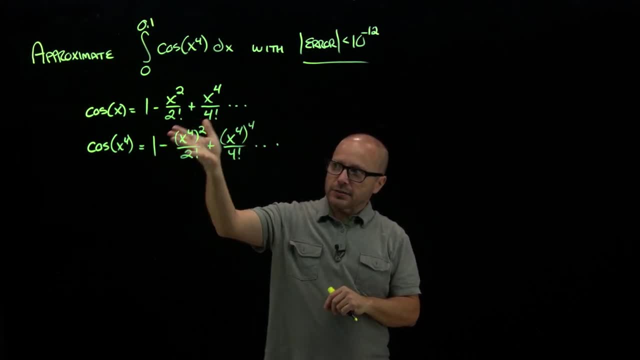 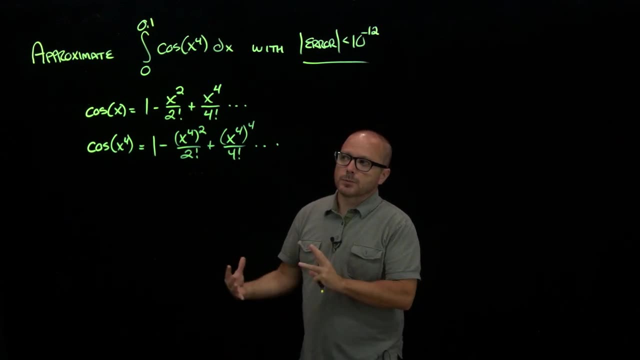 for right now. I'm just kind of writing out the details of the first few terms. I don't know if that's enough or not, Although, to be honest with you, in the textbook homework, they are nice enough to us to not make us require six, seven, eight, nine terms Usually. 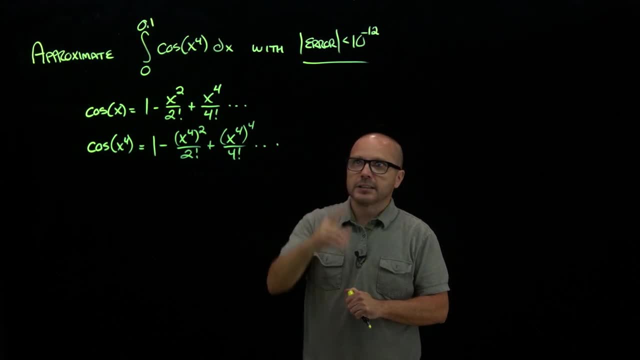 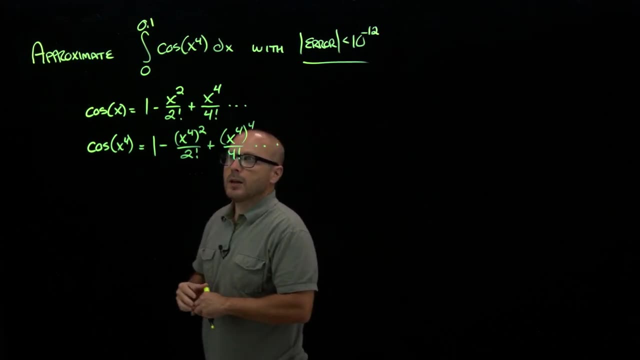 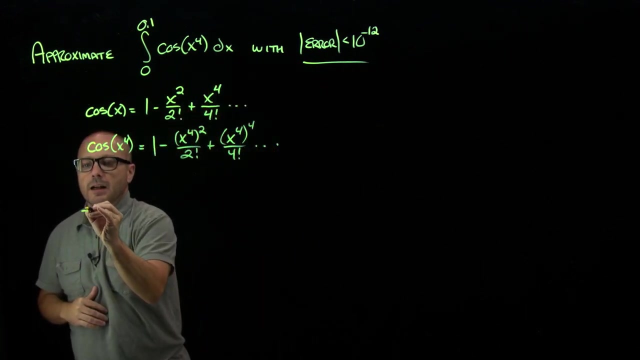 it's going to turn out that the first two or three terms is going to be enough to get the error that they ask for, So they don't punish us with a long computation. Okay, so that means that because this function and this series are interchangeable, I can say that this integral. 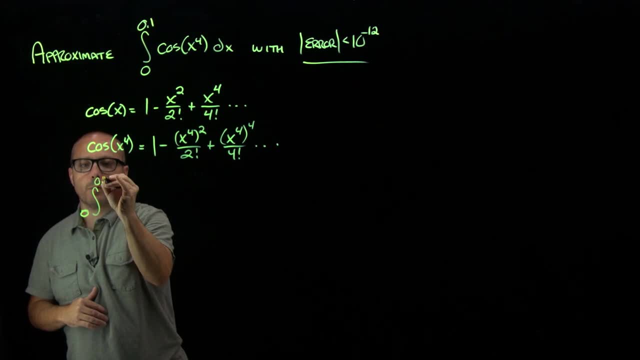 is going to be the same. So that means that because this function and this series are interchangeable, I can say that this integral is going to be the same. So that means that because this from zero to 0.1 of cosine x to the fourth is identically equal to the integral from zero to 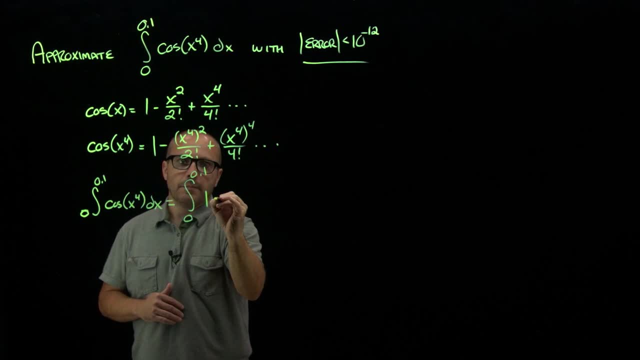 0.1 of that, One minus x to the, and I'll go ahead and simplify those exponents and those denominators: Four factorials, 24, and so on. Now, because I've got the dot, dot, dot, that's. 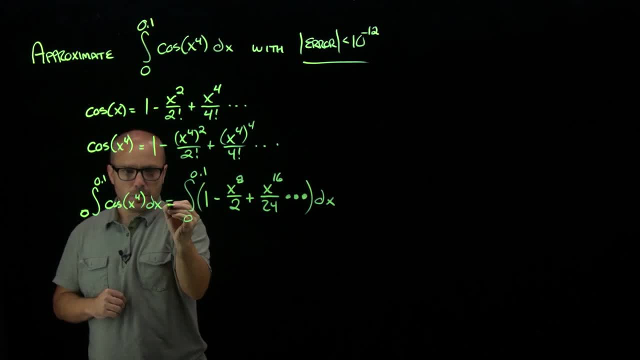 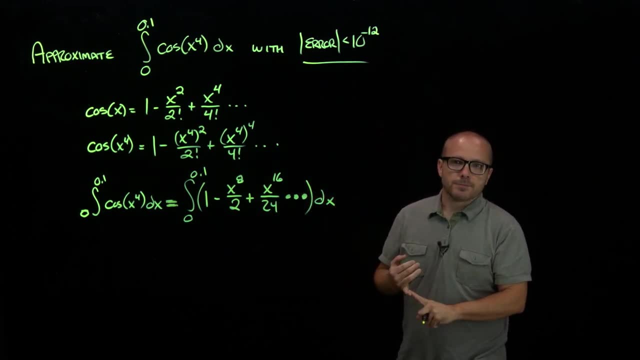 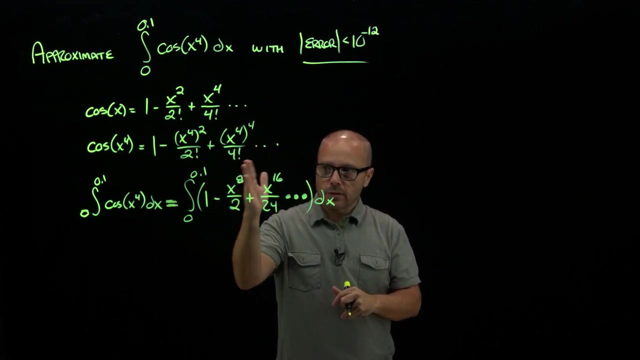 implying that that's the entire series. right? So there's no approximation yet That's an equal sign there. Those two things are identically equal. Now, term-by-term integration theorem put to use. now We know how to integrate this thing. We just go through and integrate the terms. 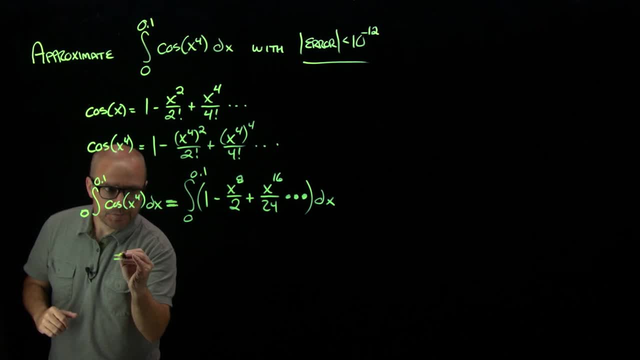 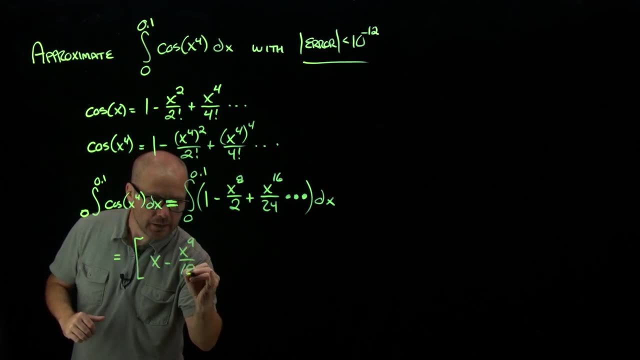 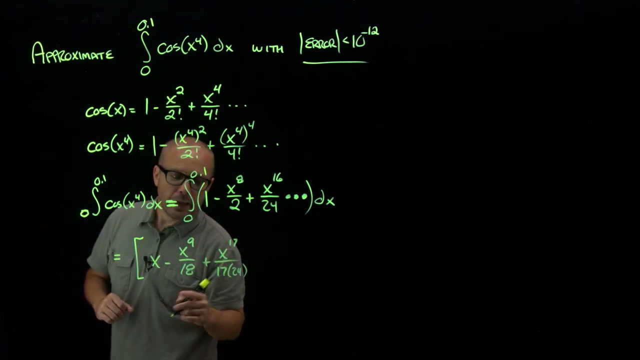 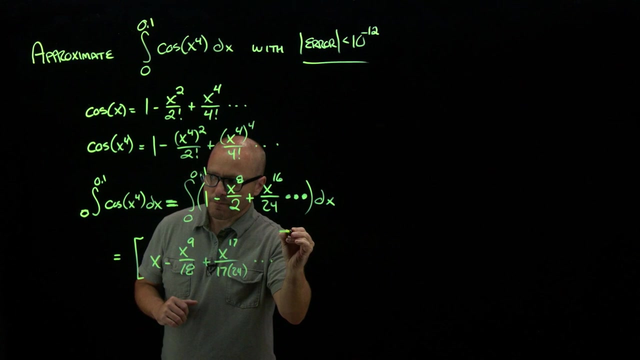 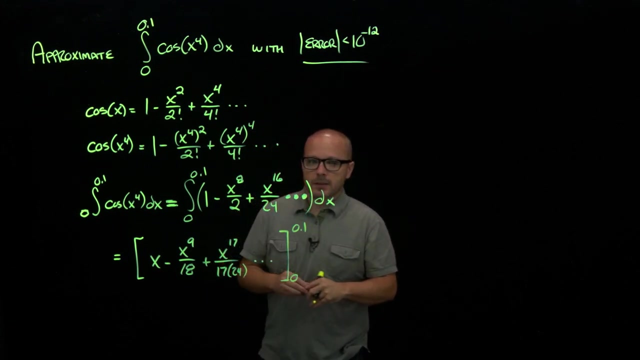 So this should be equal to x minus x to the ninth Over 18, plus x to the 17th over whatever 17 times 24 is, And I'm not even going to bother calculating that, And I'll tell you why in just a minute. And on and on, Okay, Notice, and I'll. 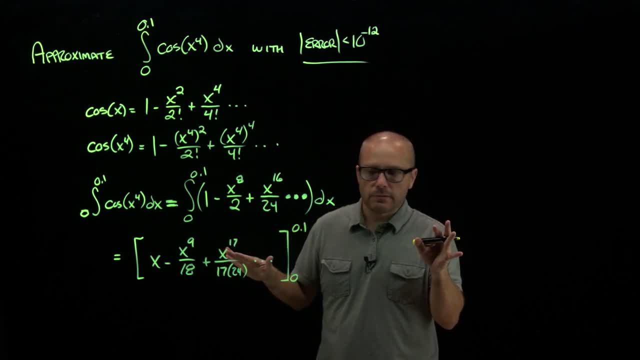 harp on this all the way through. So far, there's no approximation That is identically equal to that Term-by-term integration theorem. So that's an equal sign there. So that's an equal sign there. So that's an equal sign there, That's an equal sign. Let's start with the term integration theorem. 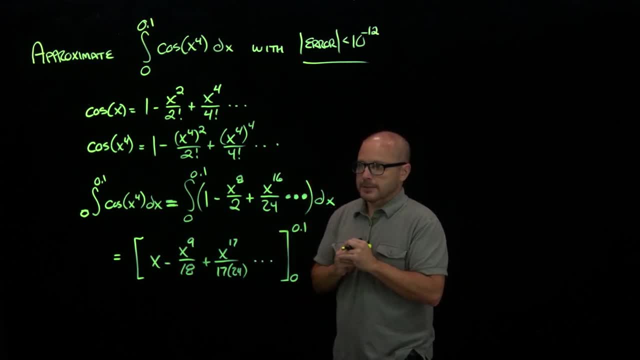 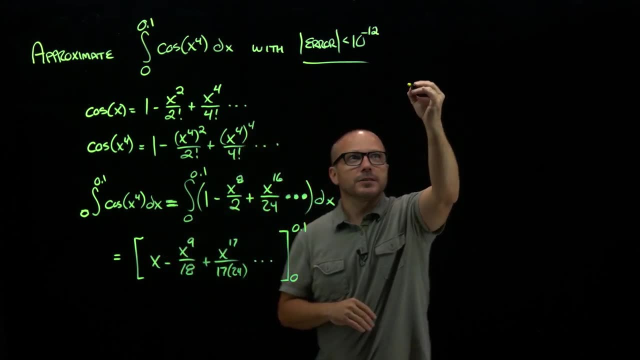 This is identically equal. There's no error yet. Now fundamental theorem of calculus. We're gonna plug in point 1.. We're gonna plug in zero. So over here I'll say that this is then identically equal to. 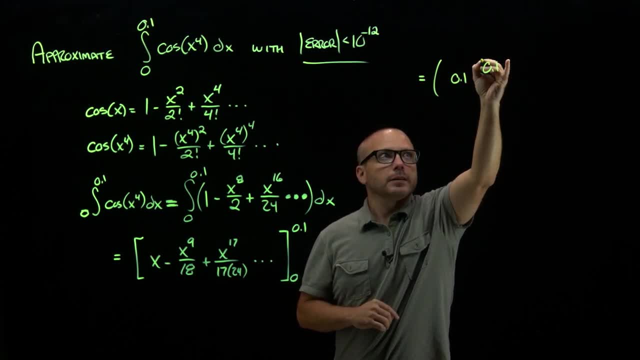 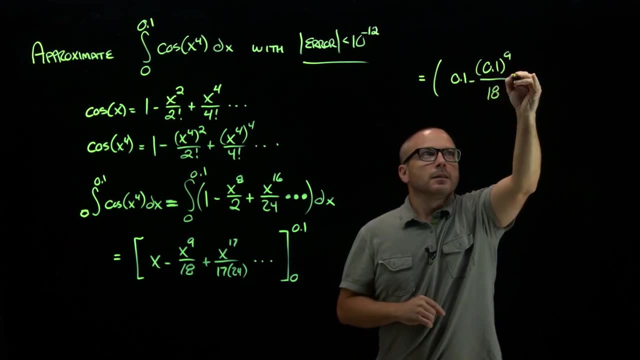 0.1, 0.1 to the ninth, over 18, plus 0.1 to the technicians And then plus 1 enormously. So this is the whole thing. This curve is going to be good. And so I'll say: if I do that over 18, then the plus size that is going to be the sum over the across is going to give me y to 10 to the 19th. Then I'm going. 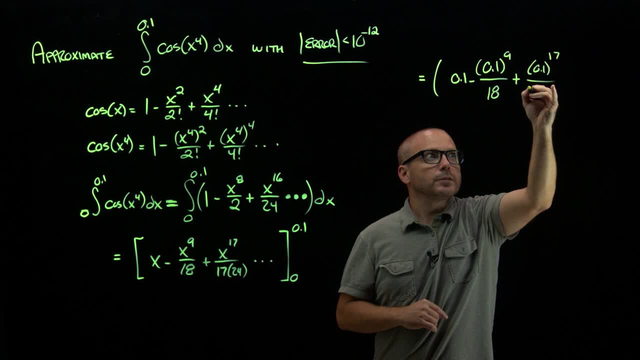 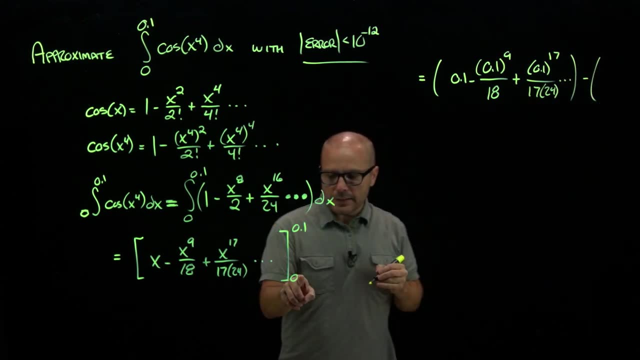 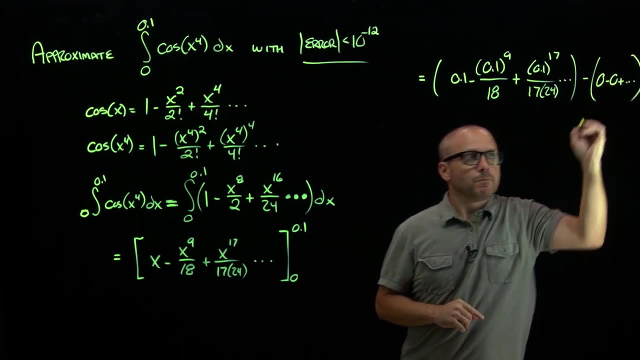 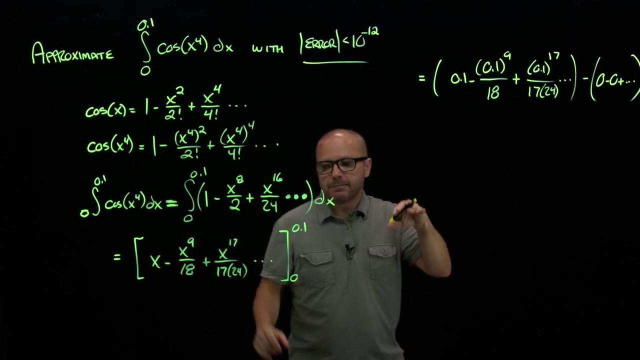 the 17th, over 17 times 24, and so on. minus now. this is nice. when zero goes in, it's zero minus zero plus zero, and so on. Now, still equal right Because of the dot, dot, dot. this is. 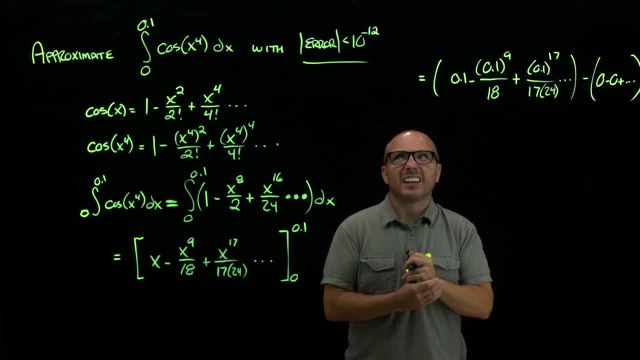 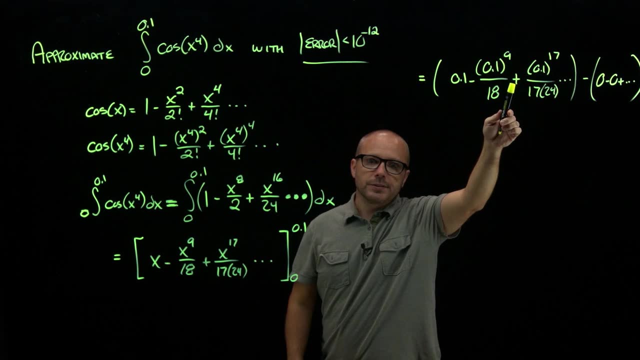 identically equal to that. Now we have to approximate. That's where our error bound comes in. Now notice: this is an alternating series, So I'm going to use alt series error estimation theorem. Remember that says that my error bound is always less than my next term or my next u. 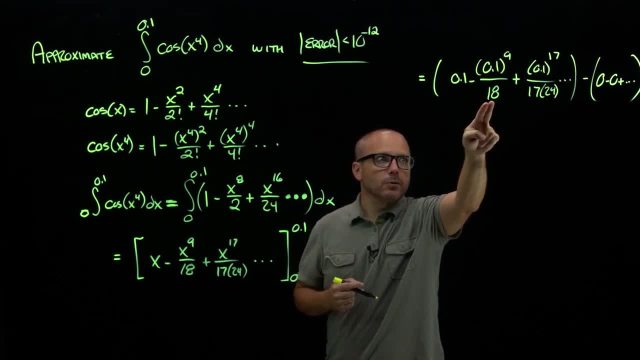 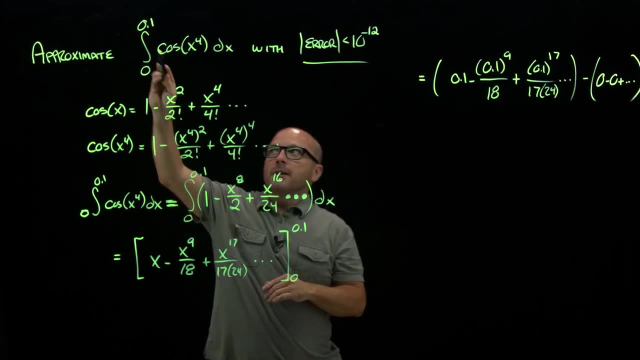 so ignoring the plus minus. So what I want to do is search through here until I reach the first term, that's less than 10, to the negative 12th, And there's a there's. there's a method to our madness here, of using this as an upper limit. This makes 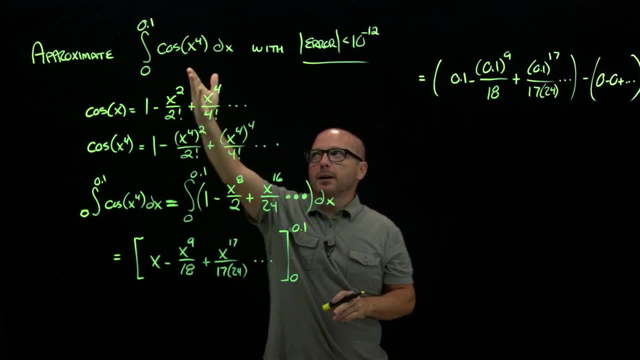 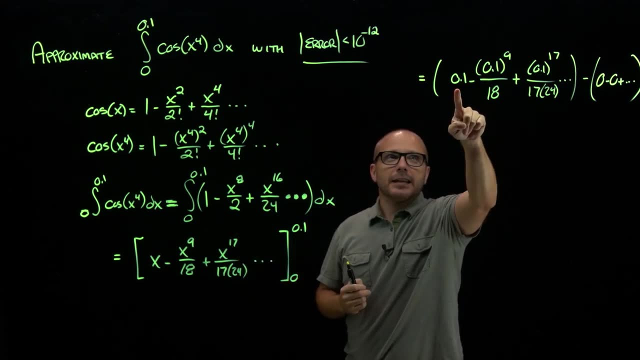 hand computation really easy. That could be any number, but making it 0.1 makes it simple, because what is 0.1?? It's 10 to the negative 1. So this is 10 to the negative 1. This is 10 to. 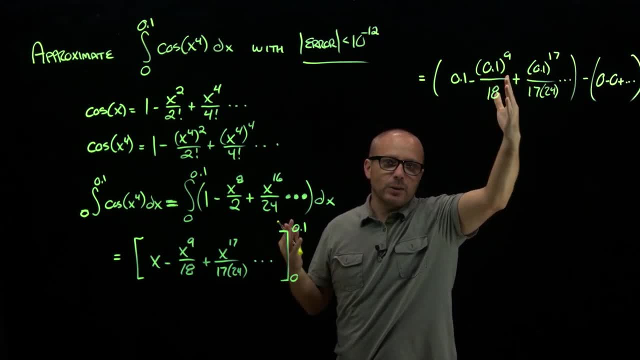 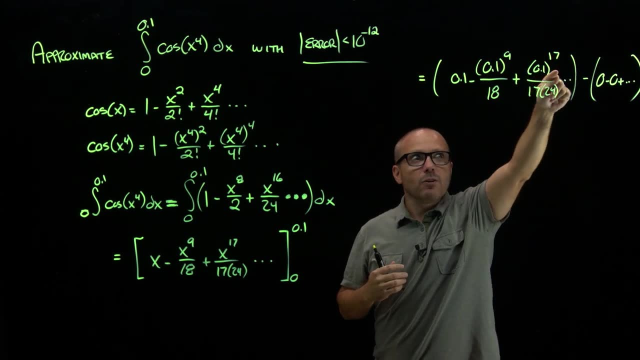 the negative 9th divided by roughly 10.. So that's in the neighborhood of 10. to the negative 10th: not quite small enough. That number on top is already 10, to the negative 17th: It's already smaller than that and it's being divided by some. 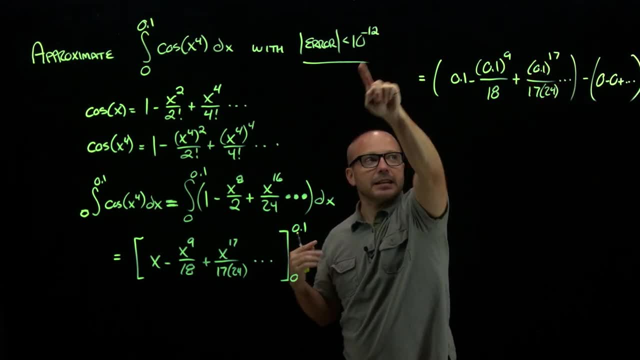 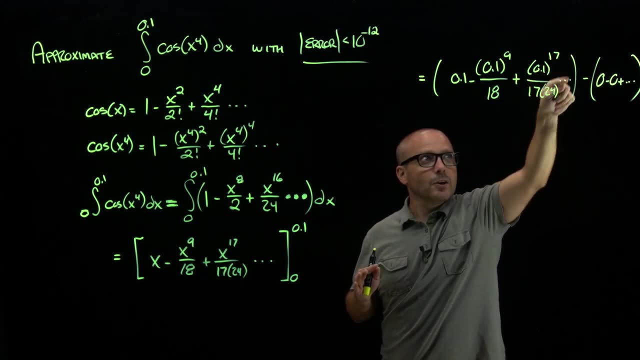 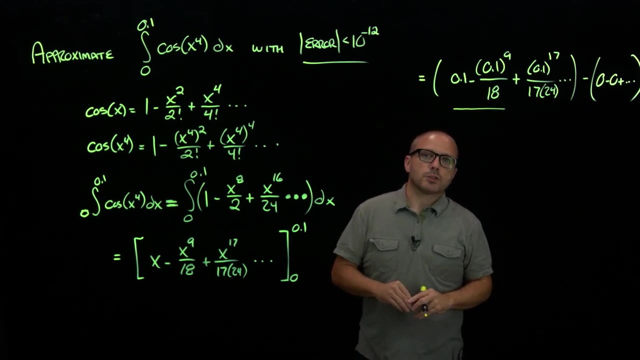 big number. So this is definitely less than 10 to the negative 12th. And now you see why I didn't bother multiplying these together. It's not going to really matter, because this term is definitely less than 10 to the negative 12th. So all I'm really going to need to use are those first two. 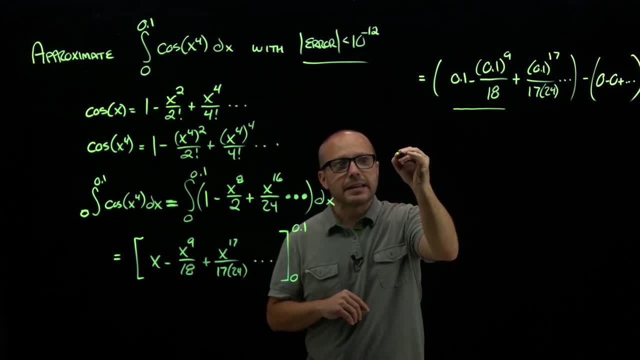 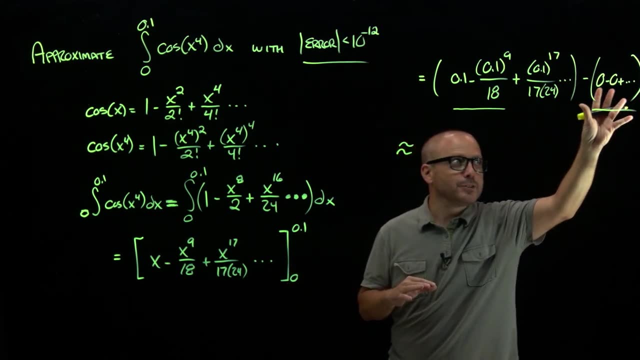 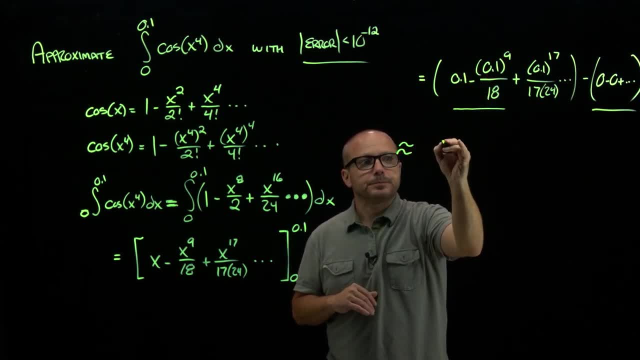 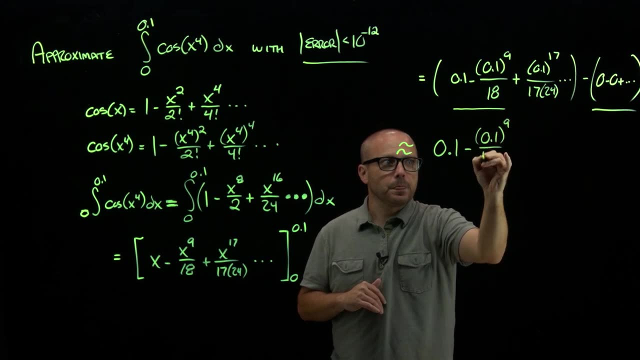 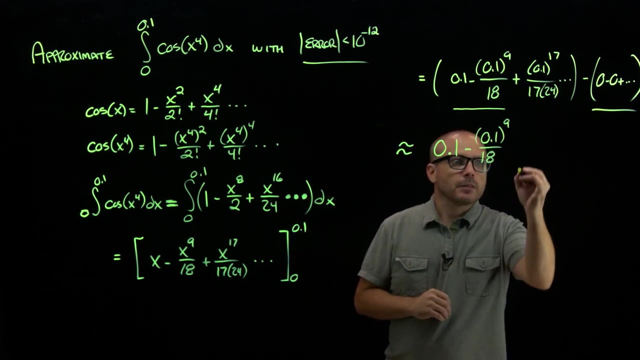 introduce error when I stop at that term. So 0.1 minus 0.1 to the 9th over 18.. And then I want to state why. I know I've achieved that error. Well, I know that my error magnitude is less than my. 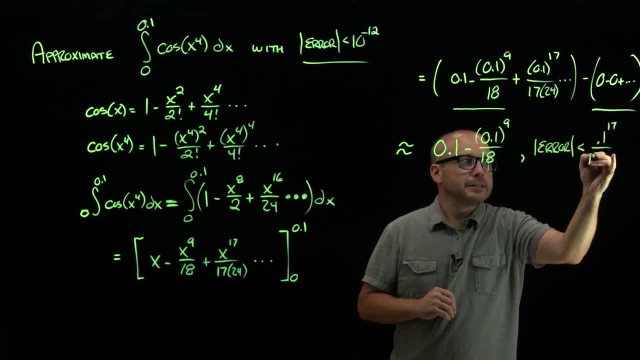 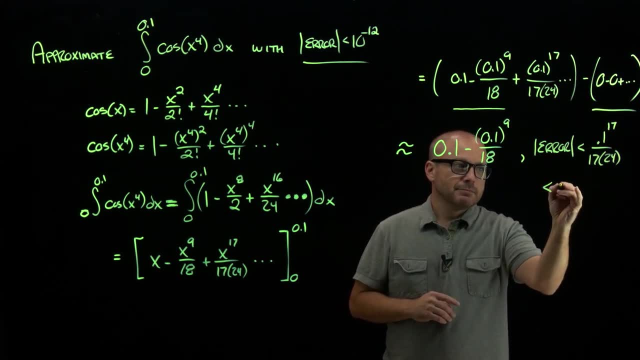 next term: 0.1 to the 17th, over 17 times 24.. But that's definitely less than 10 to the negative 17th, right, Because that's 10 to the negative 17th divided by something big, and clearly that's. 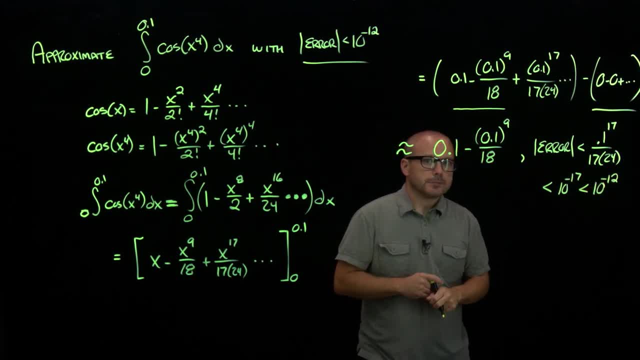 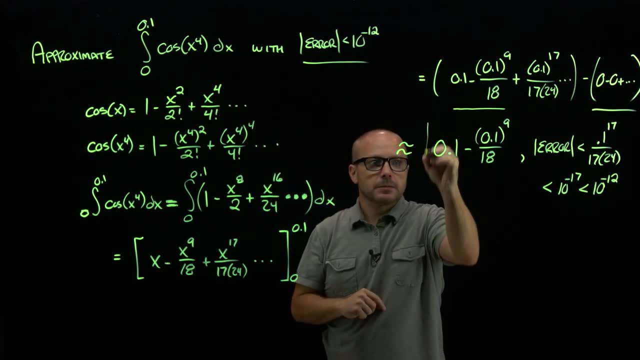 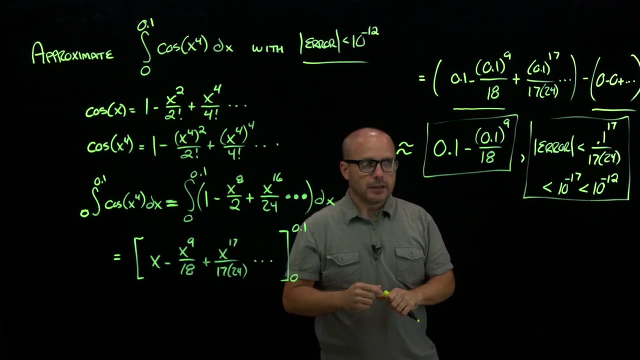 less than 10 to the negative 12th. So here's our approximation. That integral is approximately equal to this And we know our error is definitely less than what we wanted there. So I want to see both those I want to see. 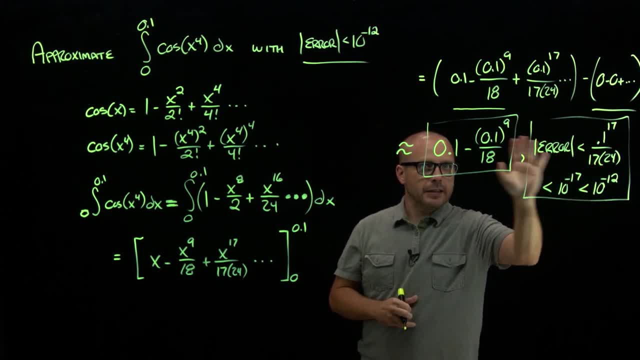 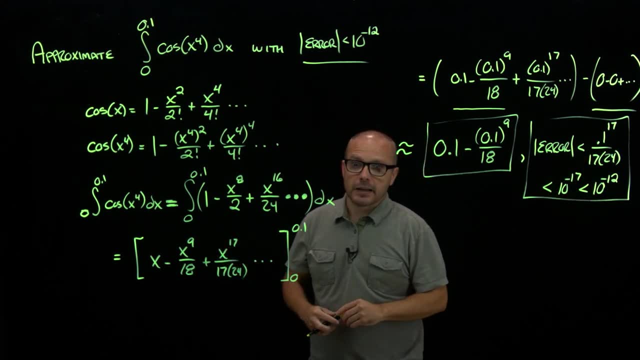 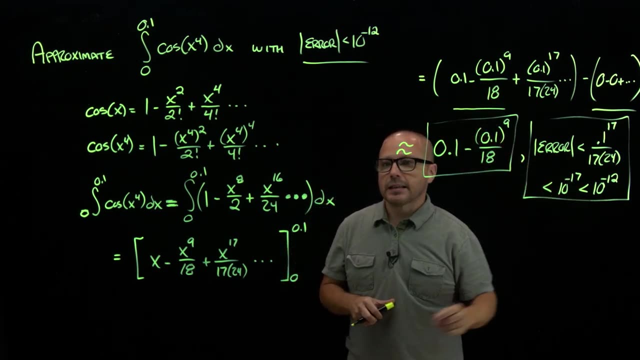 you truncate and I want to see you argue why. that's what you wanted to truncate at right. Why is two terms good enough? Because the third term is less than 10 to the negative 12th And by alternating series error estimation theorem, our error with an alternating series is less than the. 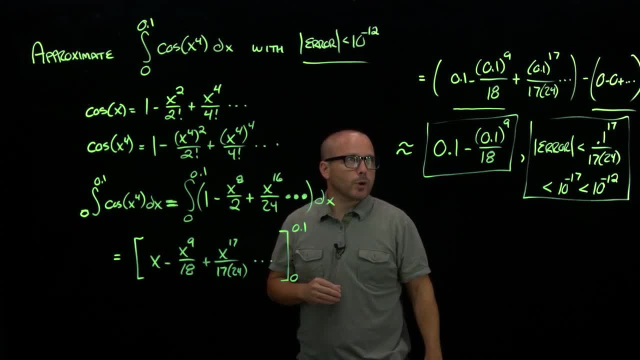 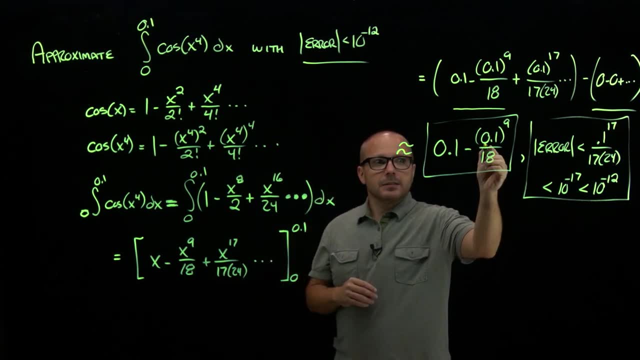 next u, which in this case was the 0.1 to the 17th over 18 times 24.. So I want to see you truncate 16th over 17 times 24.. Now the numbers in here are set up and your homework will be the same way. 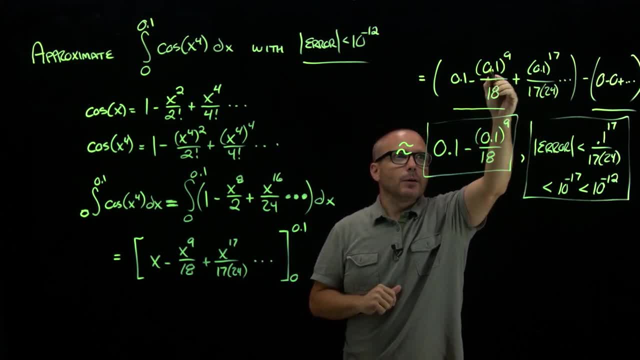 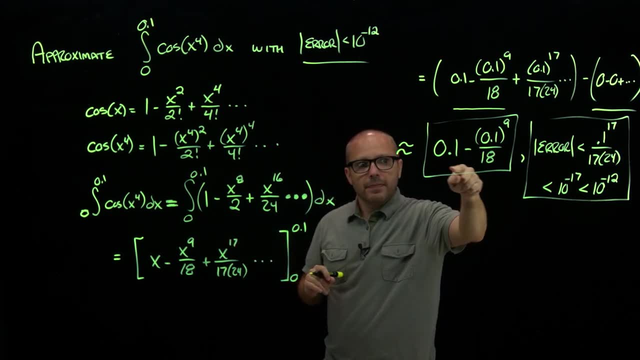 to make this easy to analyze quickly, right? I was able to analyze that this was less than 10 to the negative 12th, without really doing any computation. This might be a little tricky to finally simplify. That's why I just leave it like this. What I want to see is that you use the right number of terms. 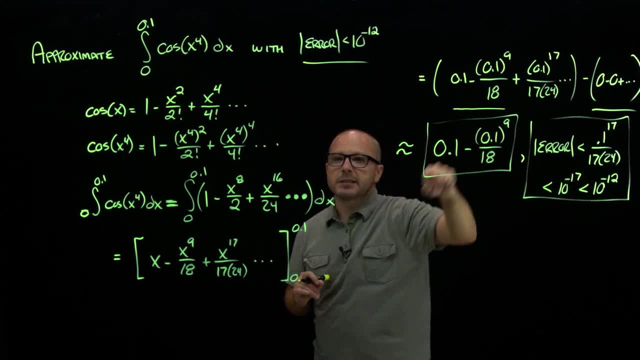 and you make it less than 10 to the negative 12th, And then I want to see you truncate this, make the right argument about your error, Don't worry about simplifying that expression down.